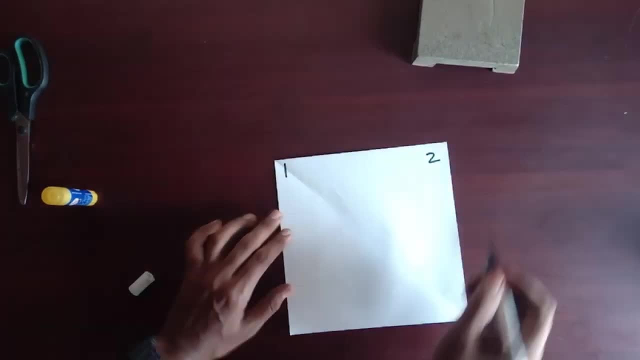 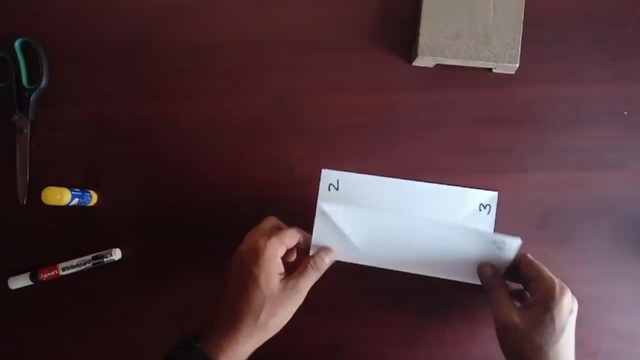 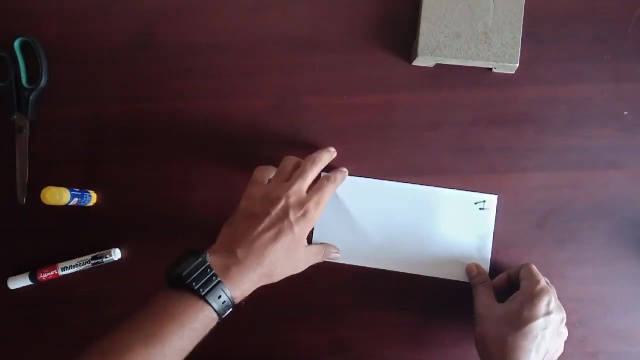 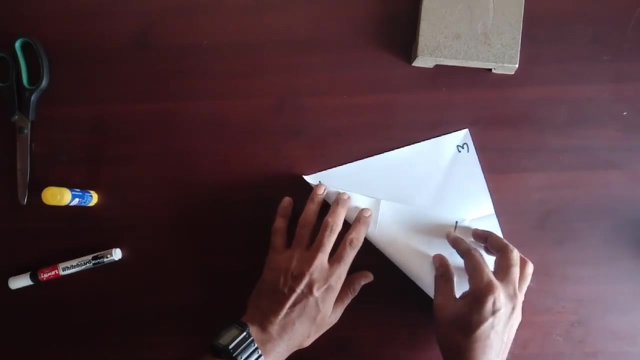 Now mark one, two, three, four at the corners. Now fold the sheet in two halves by bringing corner number one over corner number two And make the midline. Now bring the corner number one over the midline and make a fold. 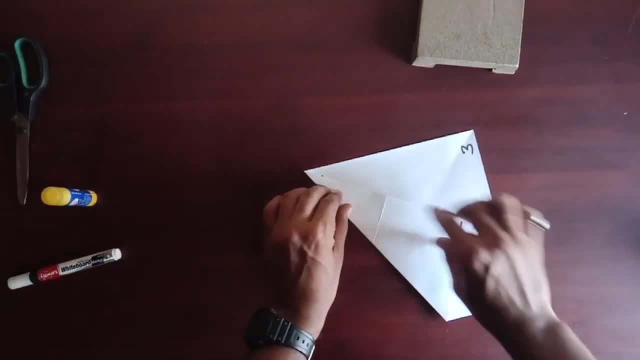 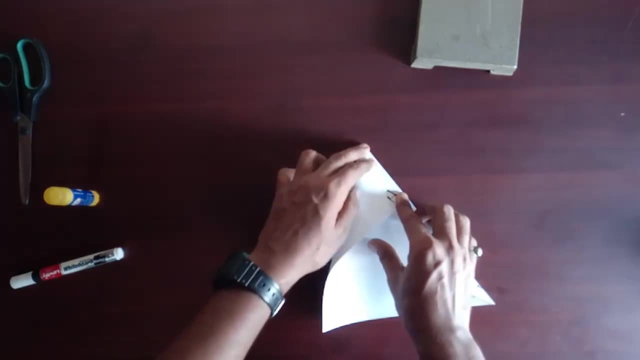 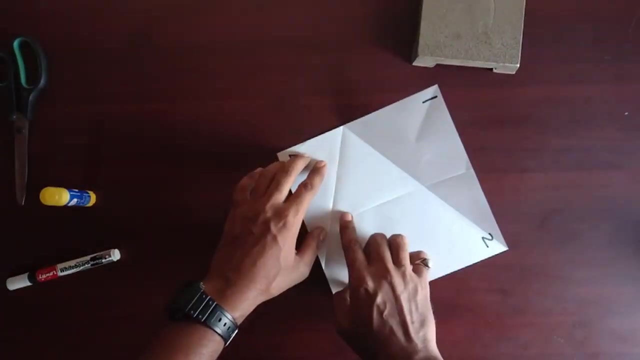 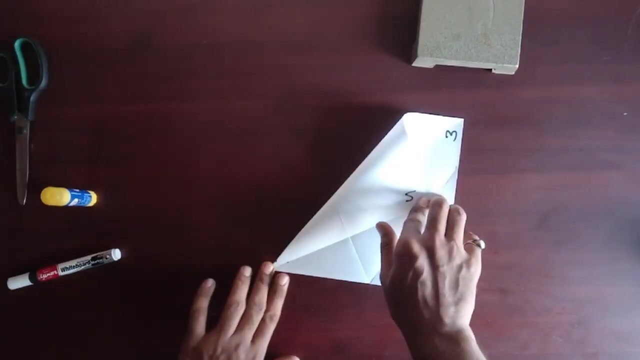 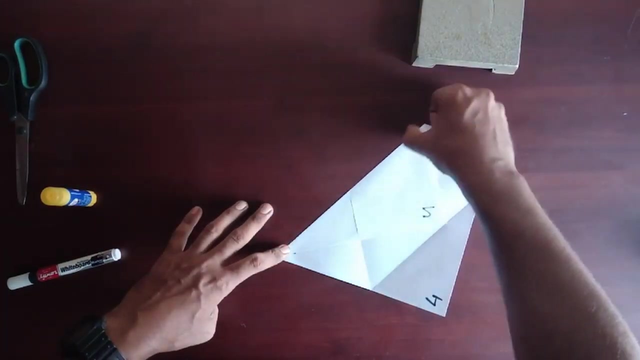 And make a fold up to corner number two like this. Now fold the corner number four over this fold and you will get a 60 degree fold. Now, similarly, bring corner number two over the midline and make a fold up to corner one. Now fold the corner number three over this fold and you will get a 60 degree fold. 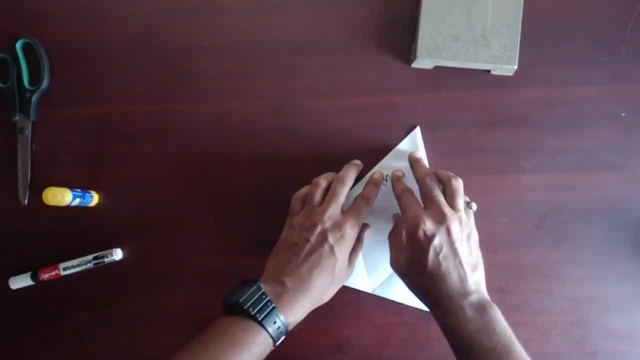 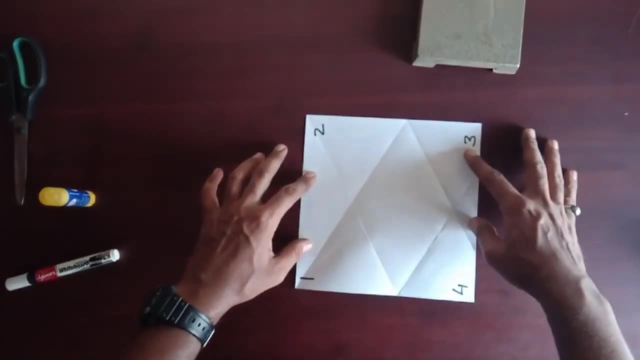 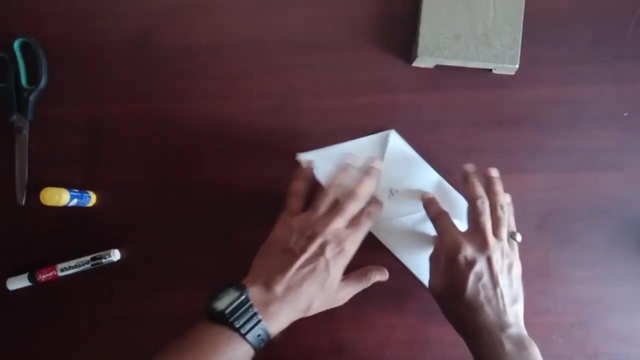 Now repeat the final part with the same mistake And fold corner three over this fold And again you will get a 60 degree angle, Only angle, 60 extent. fold up to corner number three. Now again, fold corner number one to corner number three. 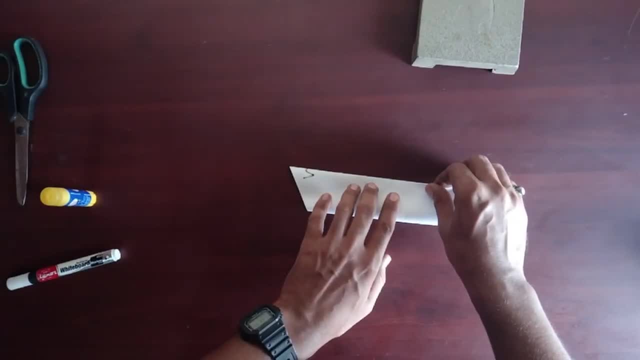 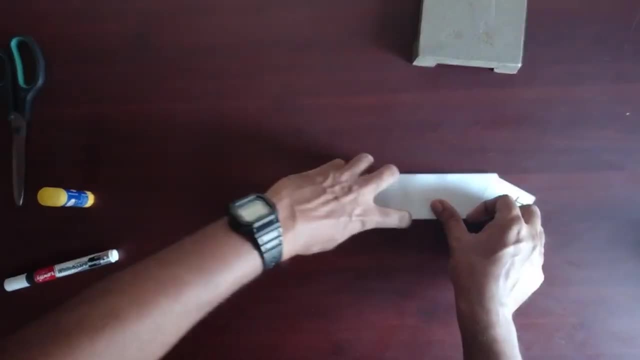 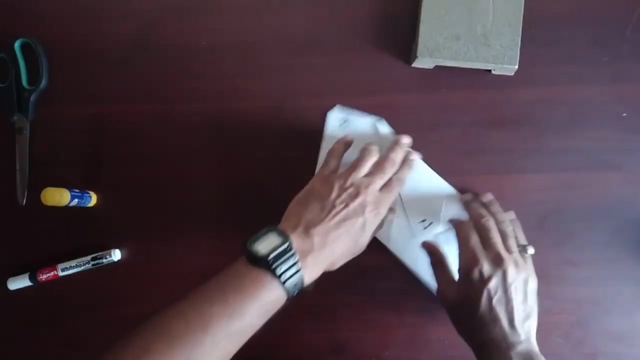 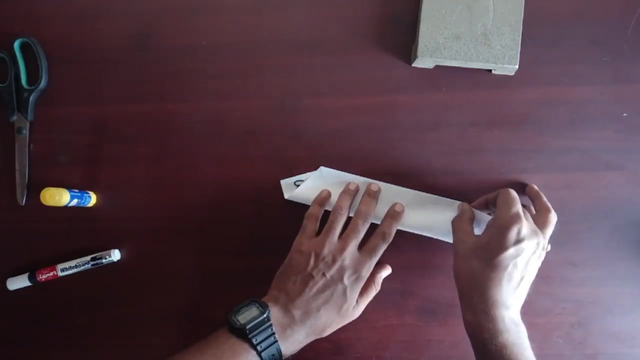 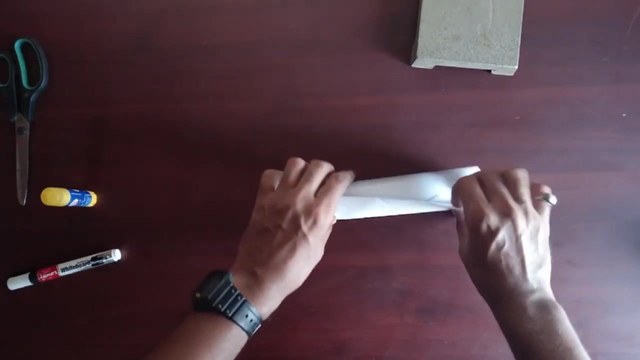 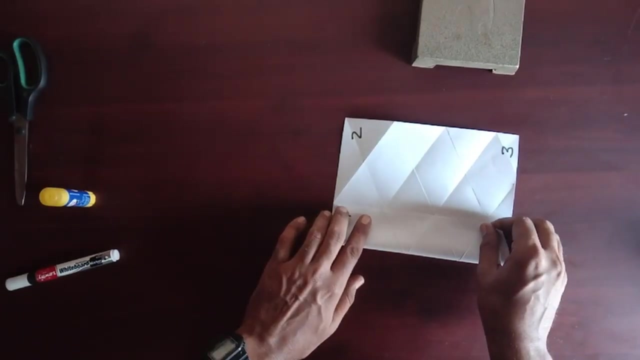 And again bed it to make a midline between them And again fold the quadrad and then fold the corner number four over the transverse angle, like this, and open the sheet and again repeat this for corner 2 and corner 4. now again open the sheet and bring the lower side over the midline and make a fold. 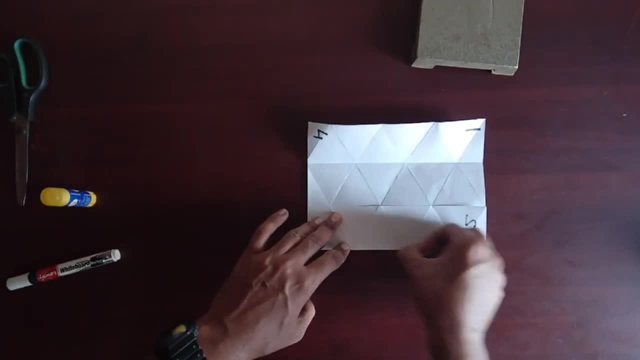 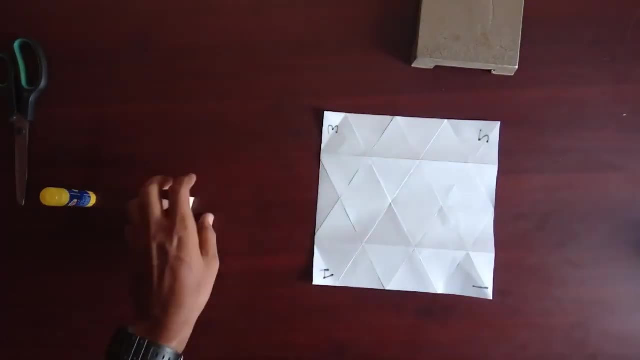 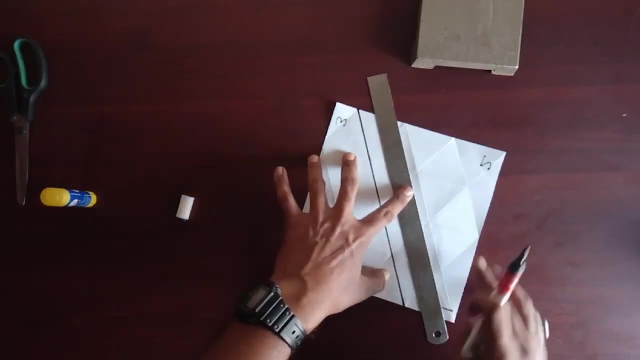 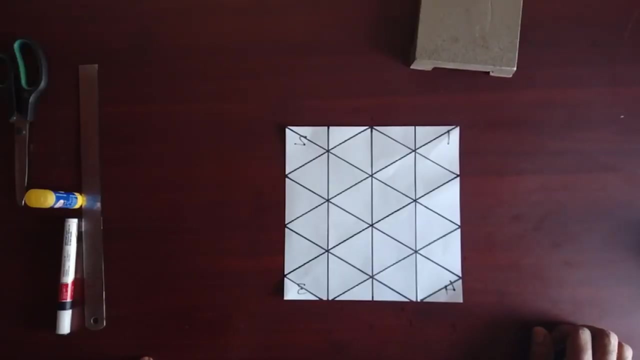 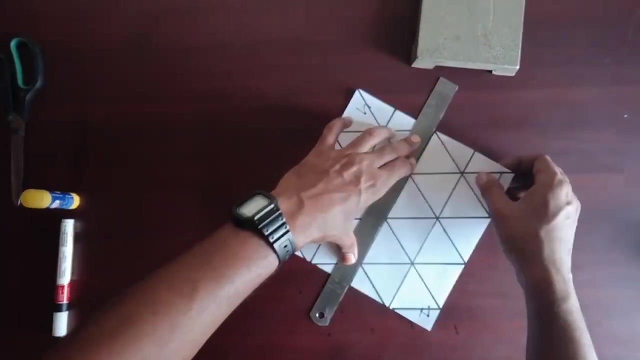 do the same for upper side also. in this way, you will see that the sheet is divided into many equilateral triangles. now highlight these folds using sketch pen or marker like this, and in this way, your sheet will look like this: now divide the sheet into two parts from the midline. 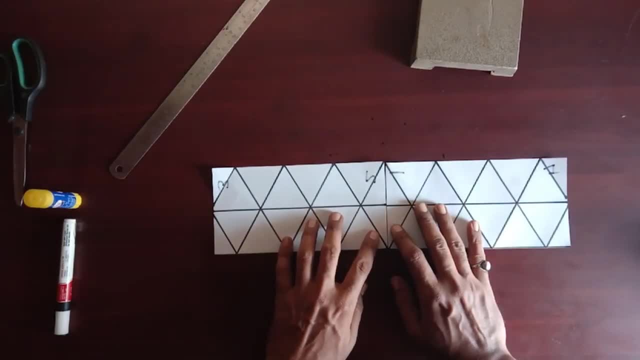 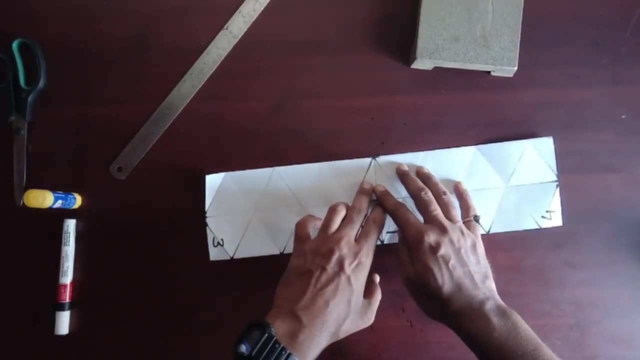 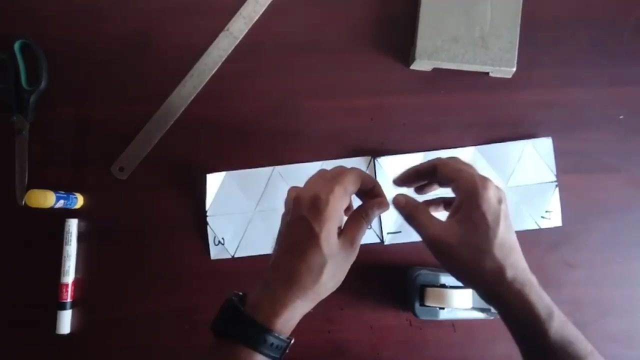 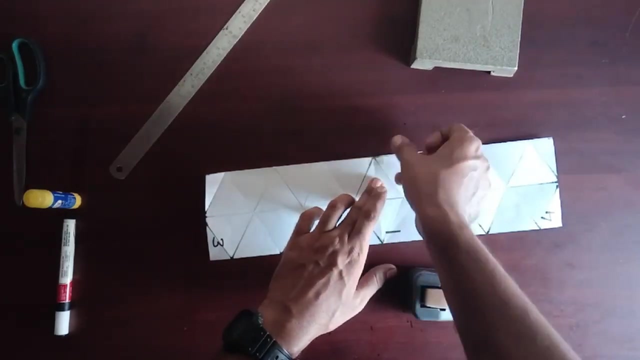 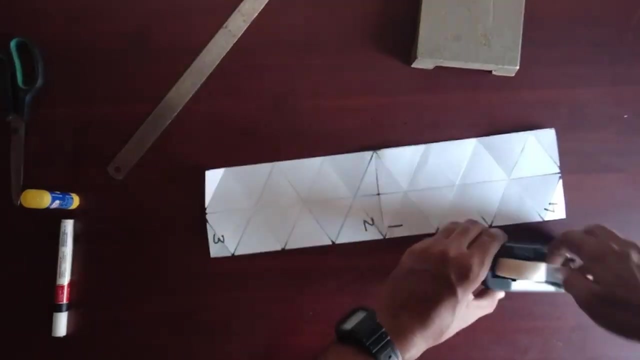 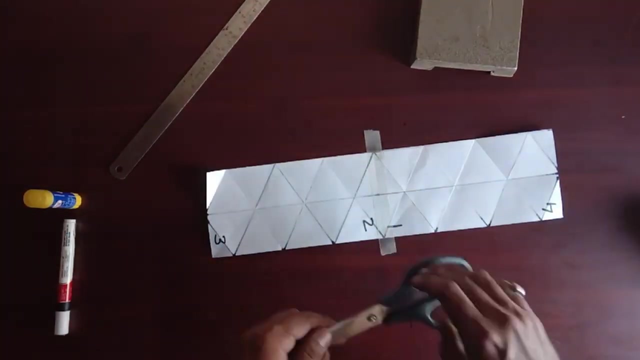 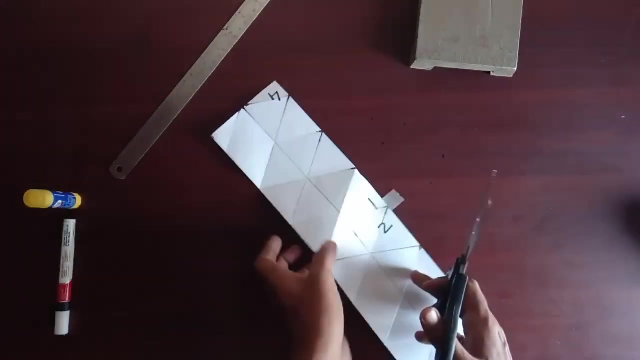 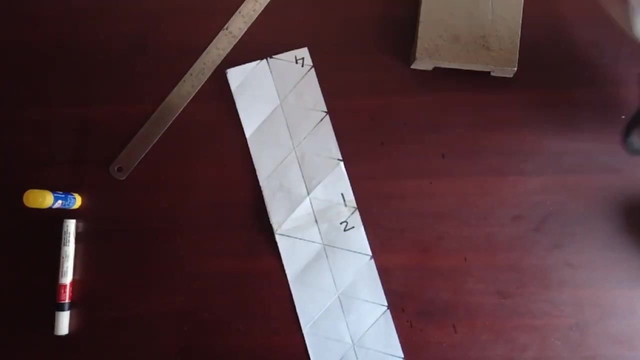 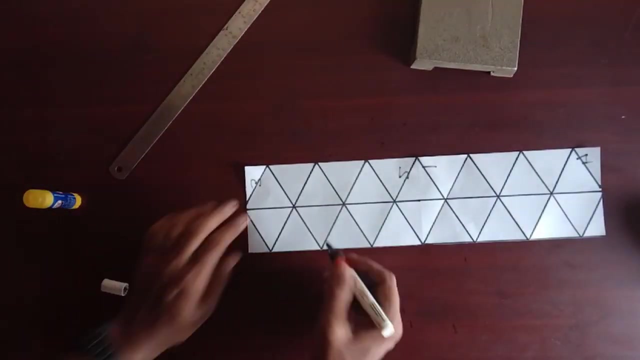 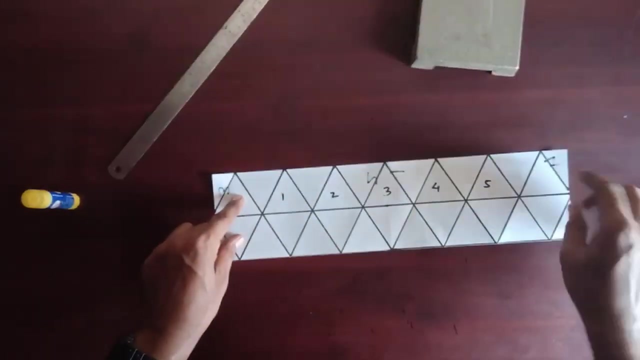 now join the both parts together and make a long strip. join them very carefully and very cleanly using tape. cut the extra tape. now in this strip, in the upper row, we need 5 full triangles pointing upward. mark them as 1,2,3,4 and 5. 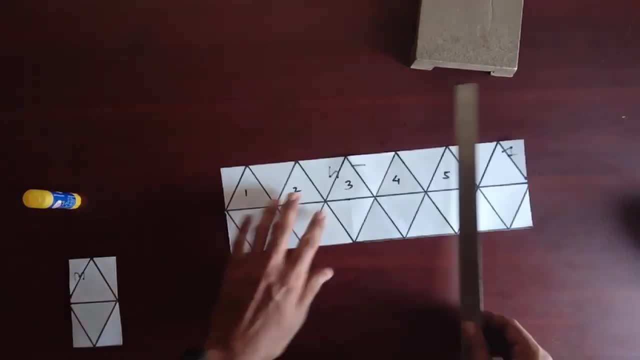 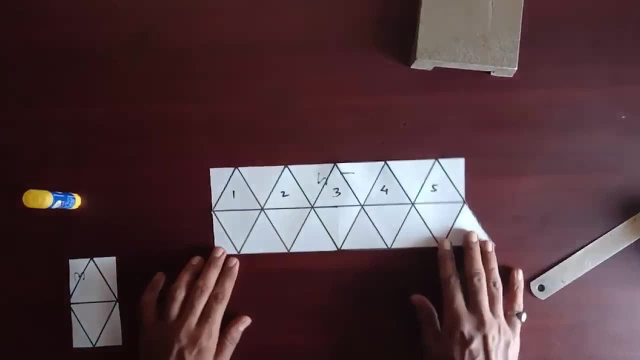 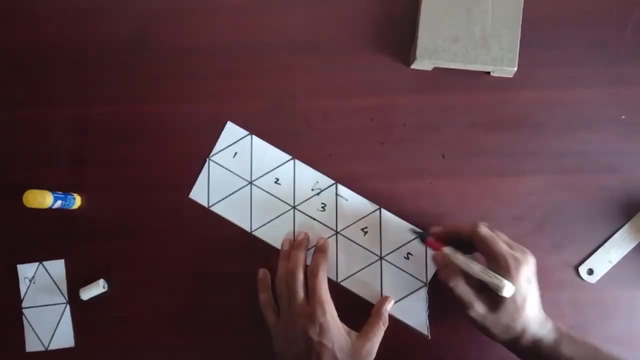 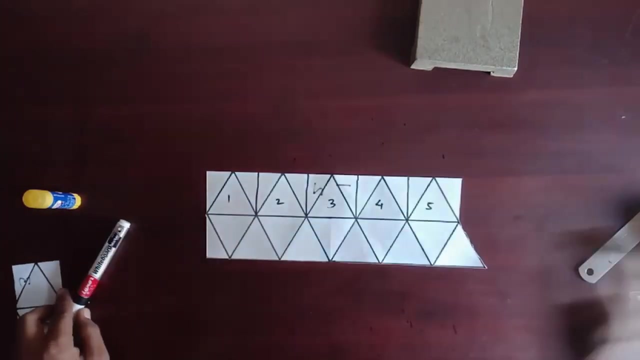 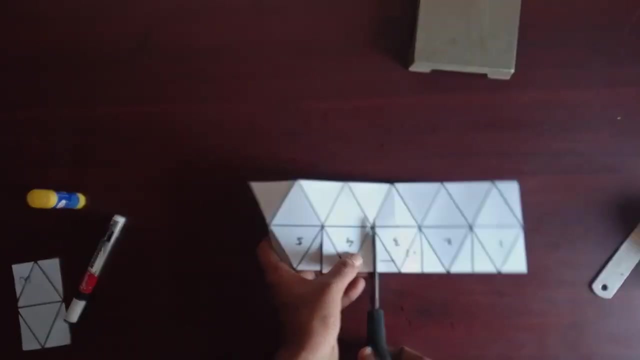 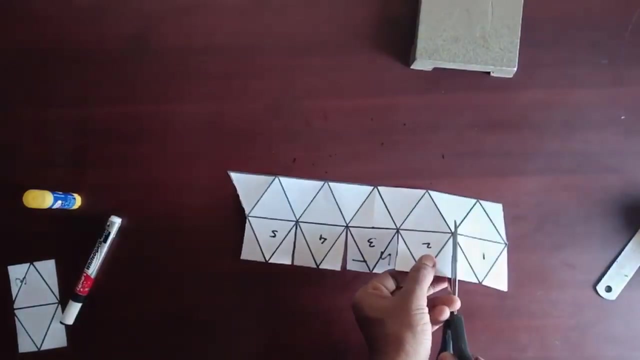 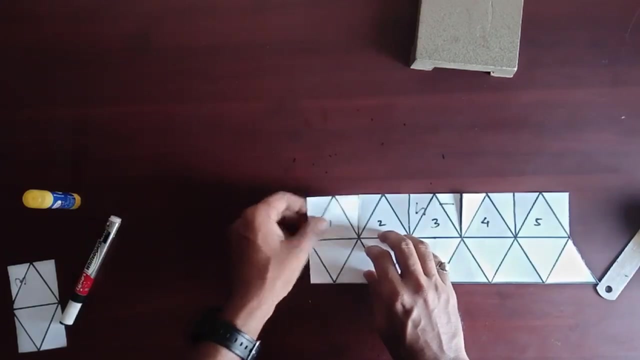 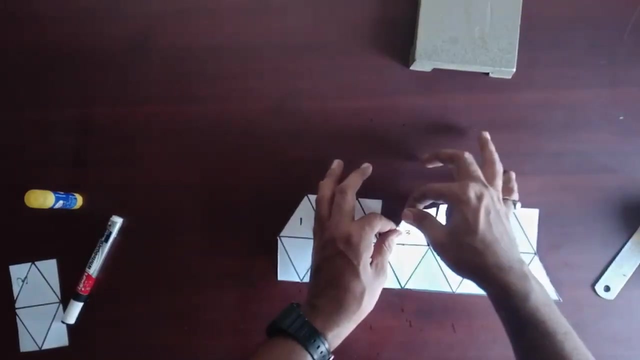 now cut the extra triangles from both the sides. cut exactly as I am cutting in this video. now separate the 5 marked triangles using scissor. separate all the 5 triangles. now you can see that each triangle have 2 flaps. fold one flap of each triangle inside, like this: 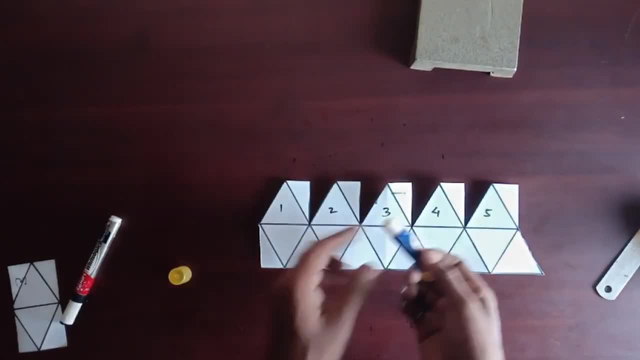 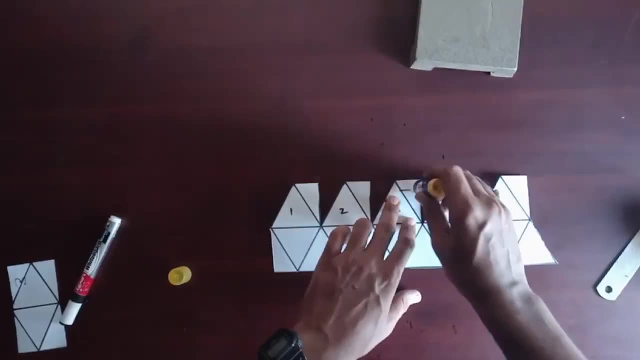 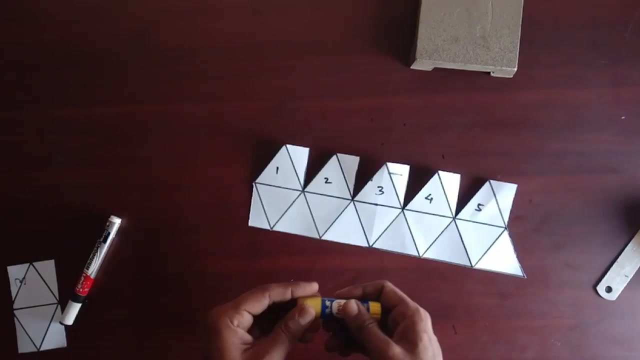 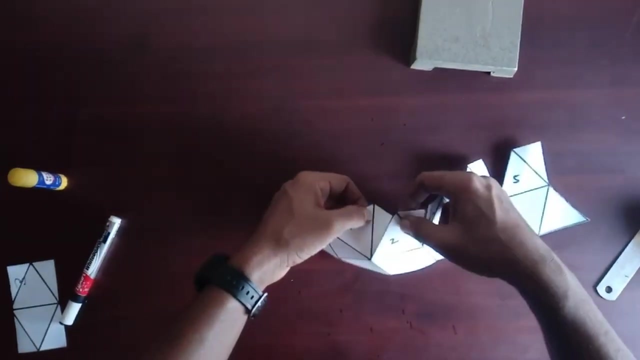 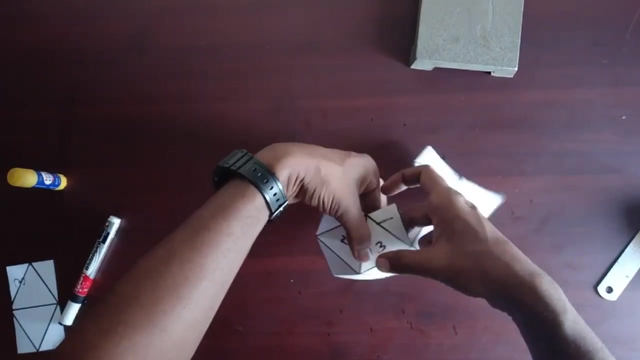 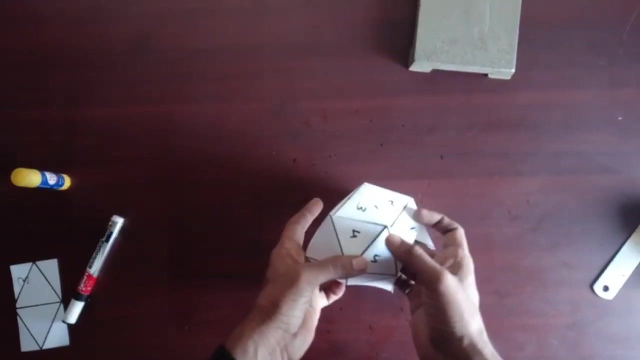 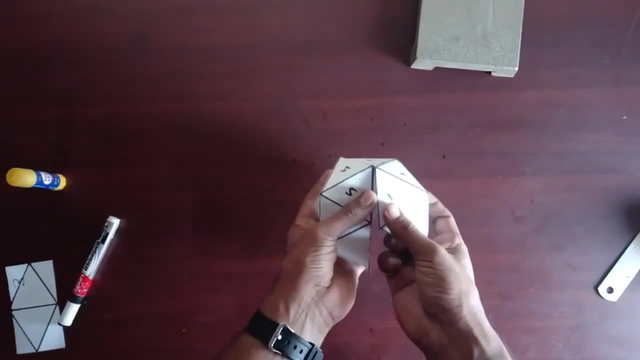 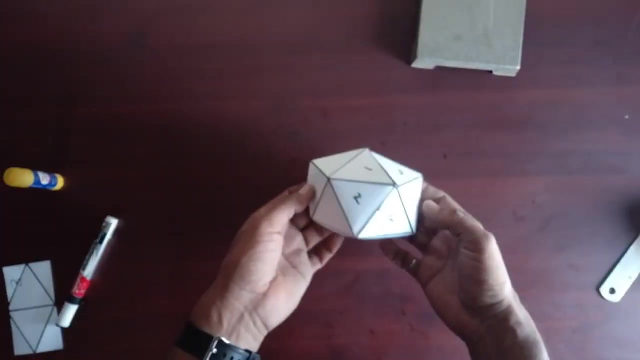 apply glue on the remaining flaps. now join these triangles with one another by pasting the flap of one triangle under the other triangle, like this: after pasting all the 5 triangles, you will get a pentagon like this. now, similarly, make one more such model.